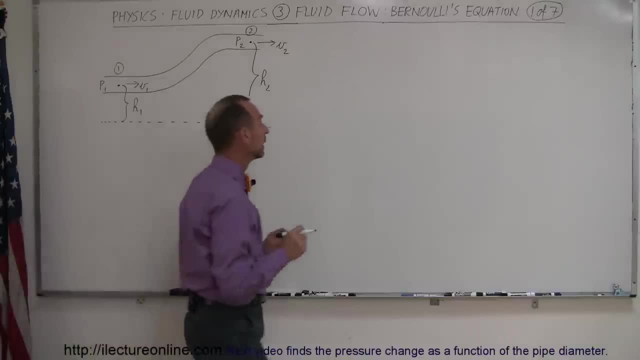 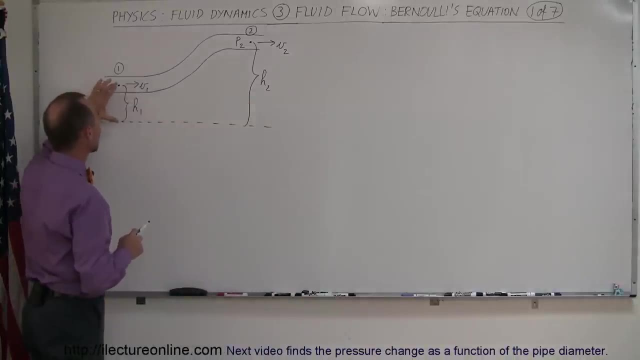 to derive the equation. but let me say what Bernoulli came up with. he took the pressure in a fluid, the velocity in a fluid and the height of the fluid relative to some reference point into an equation so that we could relate those three concepts to each other. so pressure, velocity, 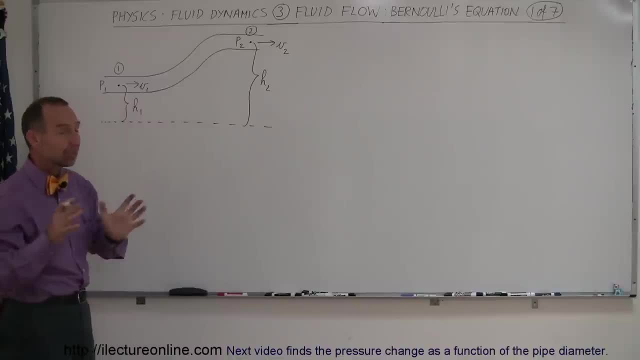 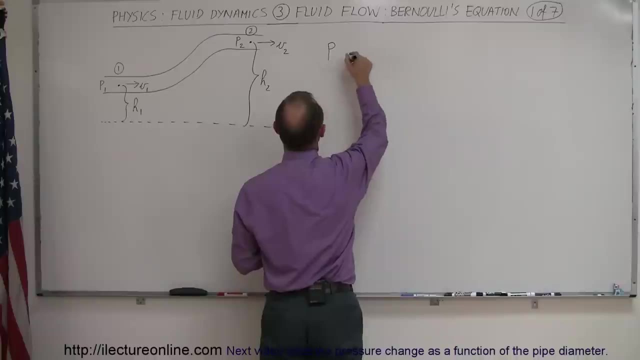 and height of the fluid. all are related to one another and he put it together into what he called Bernoulli's equation. but starting out we're going to say that the pressure at any point inside the pipe plus rho, g, h of the fluid- now rho would be the density of fluid, g is, of course, 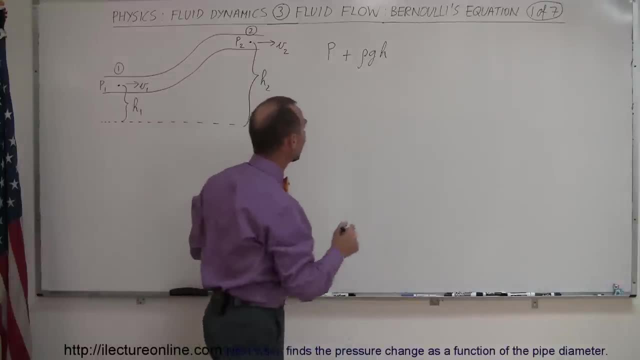 acceleration due to gravity and height is the height above some reference point, plus one half rho- v squared. again, rho is the density of the fluid and v is the velocity of the fluid through the pipe. and again, it doesn't have to be through a pipe. but for simplicity let's start. 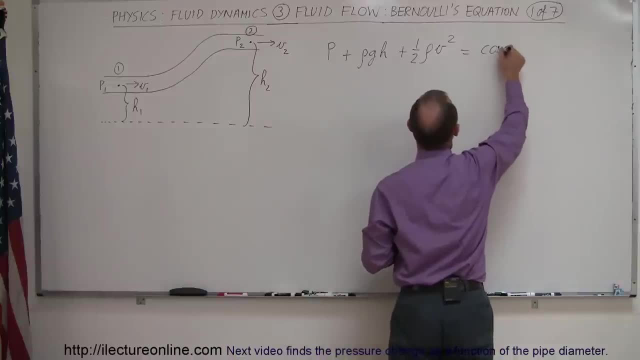 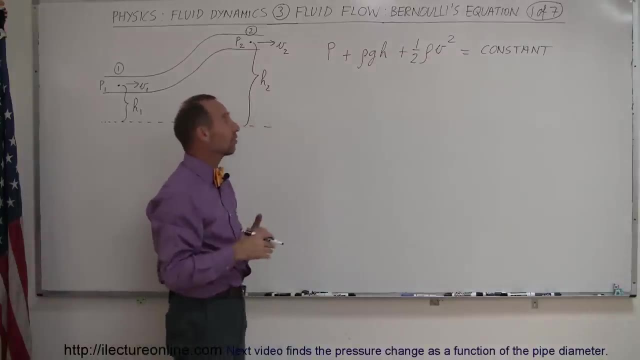 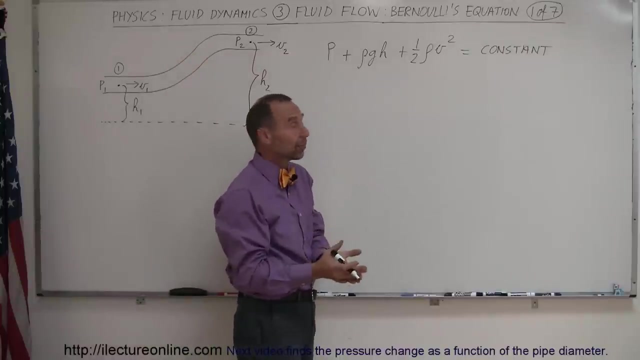 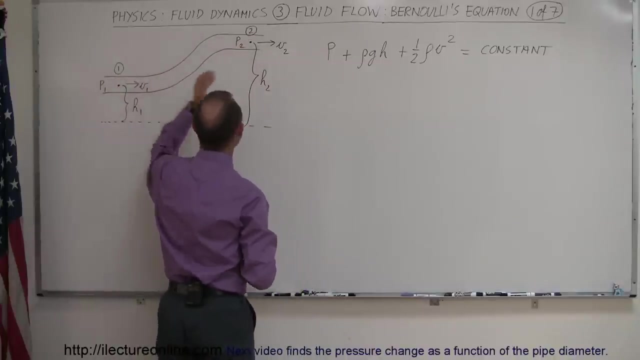 there, and he said that those three terms combined are always constant. so the velocity at point one must be equal to the velocity at point two, which means that if one increases, something else has to decrease. for example, when the pipe gains height, so that this term becomes bigger, something else has to become smaller. now, in this particular case, since the pipe 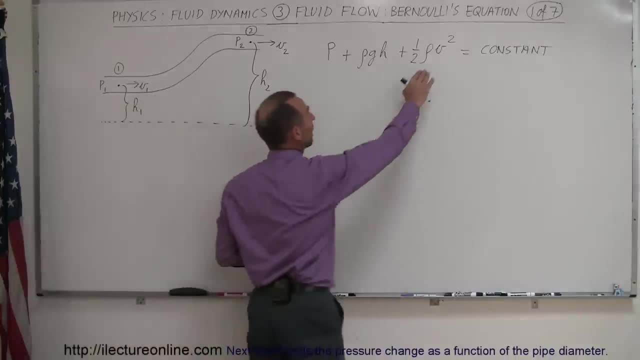 doesn't change in diameter. the velocity at point one must equal the velocity at point two. so we know that that must be the same, no matter what. and since this will increase, the only other option that we have is that the pressure then will decrease over here because of its increased height. so that's. 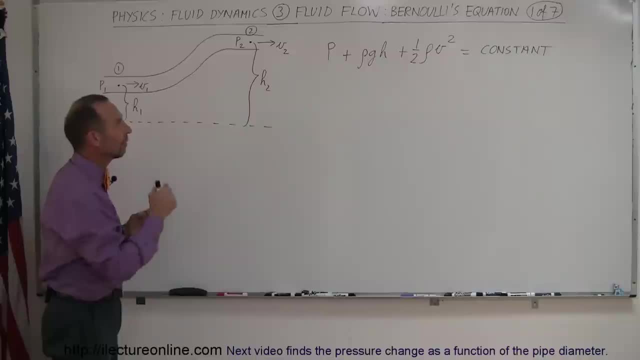 how Bernoulli was able to manipulate what happens in fluid flow. now let's make, let's write down the equation. so at point one we could say pressure at point one plus rho g, h at one plus one half rho v at one squared must equal, since it's constant, to these three terms combined at. 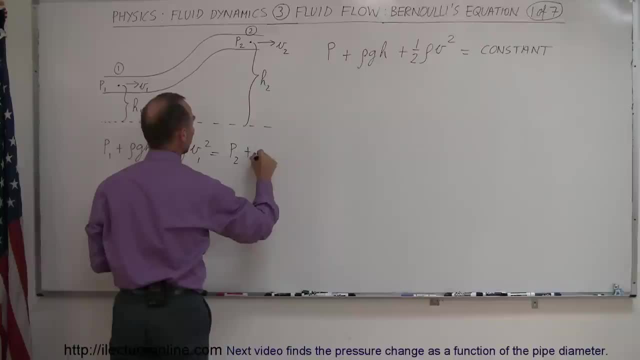 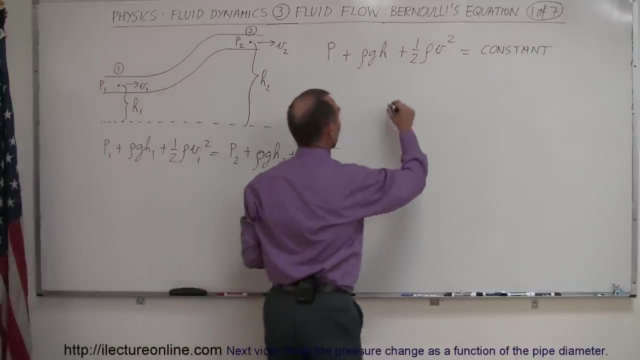 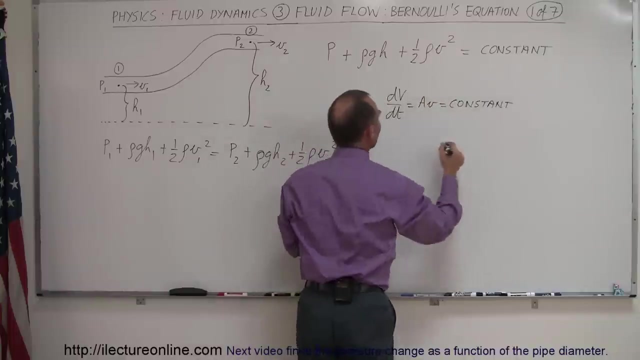 point two. so we could say: pressure at two plus rho, yeah, rho g h at two plus one half rho v two squared. now, in this particular case, since the diameter of the pipe doesn't change and we know that dv, dt, which is equal to a times v, must also be constant and therefore we can say: 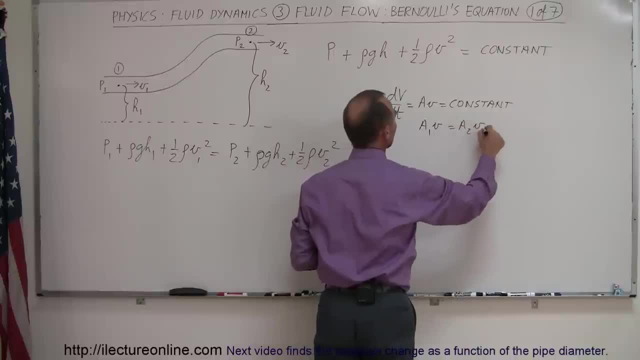 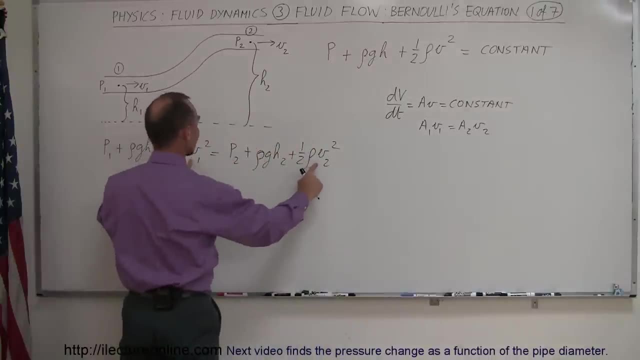 that a1, v1 must equal a2, v2, and if a doesn't change, then v cannot change. so that shows that the velocity must be the same over here and over here. so that means this term and this term are constant. they don't change in this particular example, of course, which means that 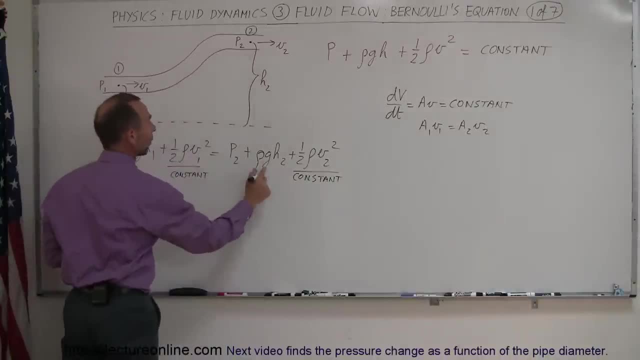 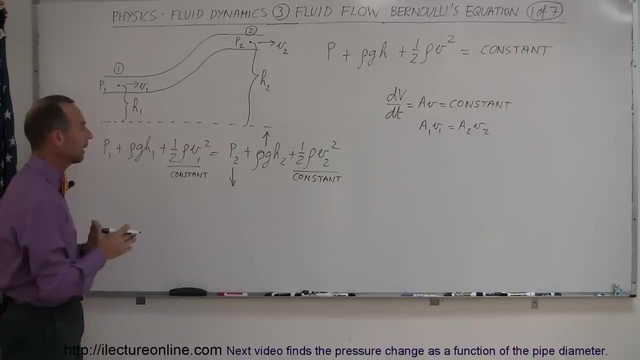 if the height increases, that means that here rho gh2 has increased relative to rho gh1. that means, in order for the equation to balance, that the pressure at two must be less than the pressure at one, and that's how you have to read that equation. that's a good way to take a look at. 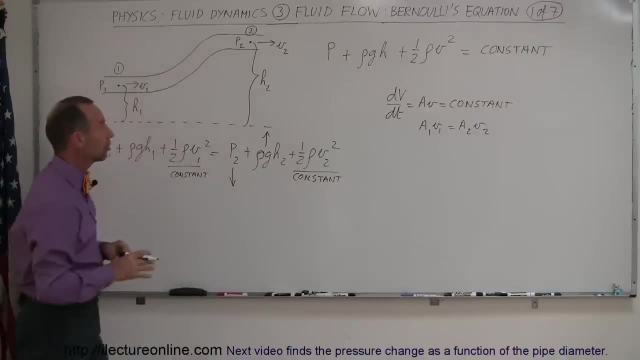 Bernoulli's equation, when only the height changes and nothing else changes, and of course because of that the pressure has to change as well. all right, now let's do an example. let's say that this height is equal to five meters above the reference point, and this height is equal to: 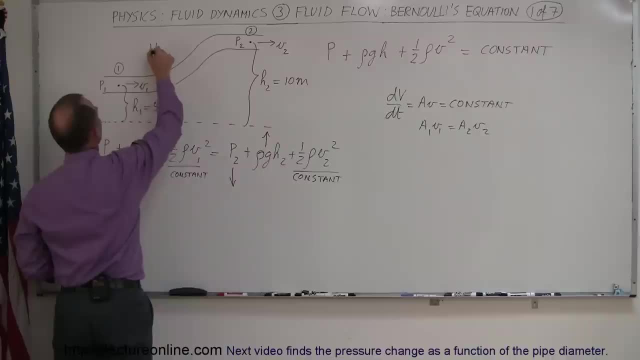 10 meters above the reference point. let's say that the fluid is water, h2o, and let's say that the velocity in the pipe is equal to two meters per second. and the question that would be, given the change in the height, given the velocity here and, of course, the velocity of the pipe, 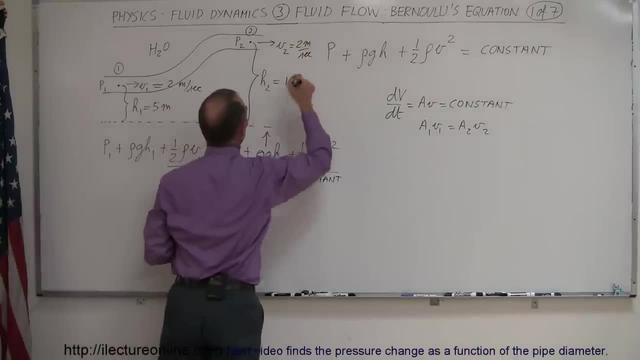 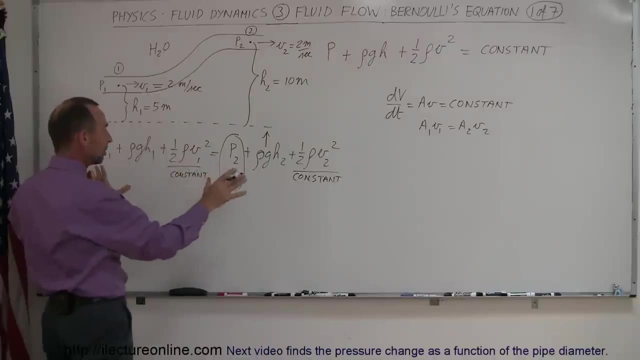 is equal to two meters per second and, of course, knowing that the velocity there also must be two meters per second, what is the pressure at the second point? all right, let's go ahead and do that. well, first of all, we have an equation. it's balanced. it's left side equals the right side. 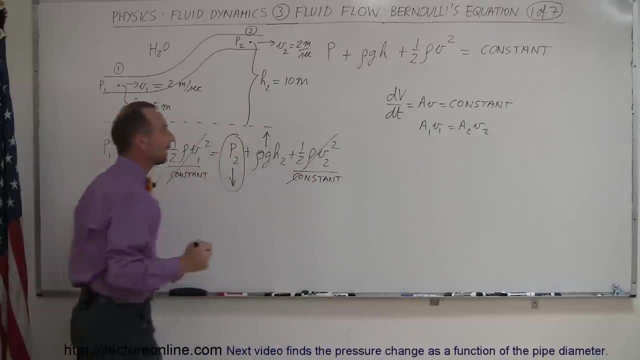 and since this is constant- that constant, it doesn't change- we can simply get rid of that part in our equation. now. solving that for p2, that means i have to take rho gh2 and move it to the other side, and of course i can then flip the equation around, which means that the pressure at point two 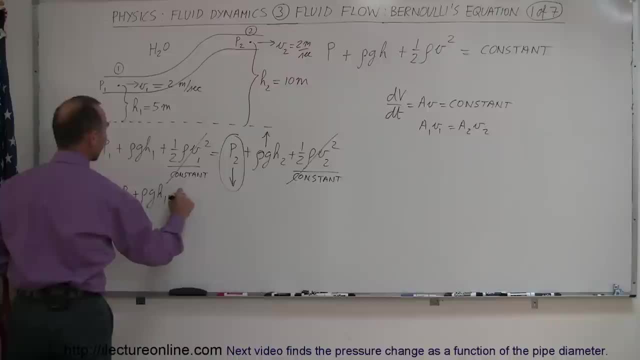 is equal to rho gh1 plus rho gh1 minus. when i bring this across, that would be rho gh2. simplifying that equation a little bit by factoring out a g and a g in a row, so this becomes: p2 is equal to pressure one plus rho g times h1 minus h2. now notice, i did not give you pressure one. 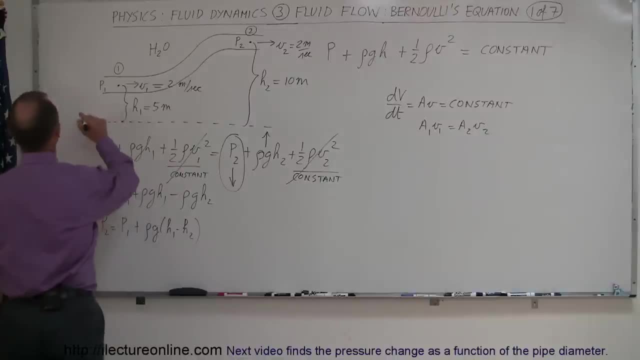 well, i can put something in there. just let's say that pressure one p1 is equal to two times atmospheric pressure, and of course, atmospheric pressure, hmm, that would be two times 1.013 times 10 to the fifth newtons per square meter. all right, so let's say that pressure. 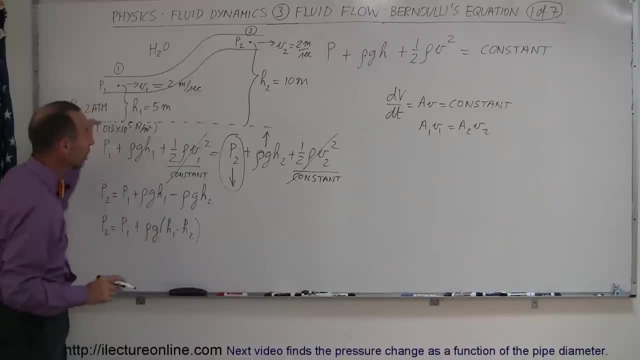 one was two atmospheres. how much will the pressure have changed by allowing the pipe to go up an additional five meters from where it was before? all right, so let's plug these numbers in. so this is equal to- i'll leave this at two atmospheres for now, plus the density of water, and of course the density of water is a thousand kilograms per. 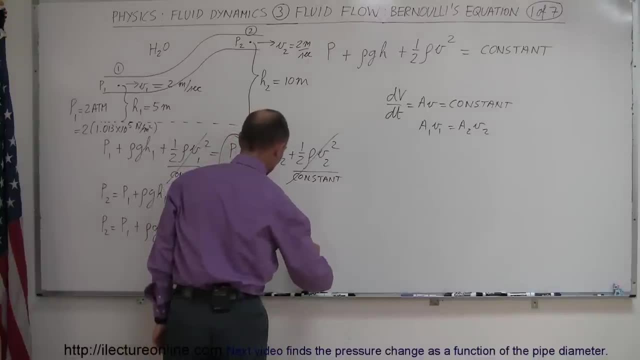 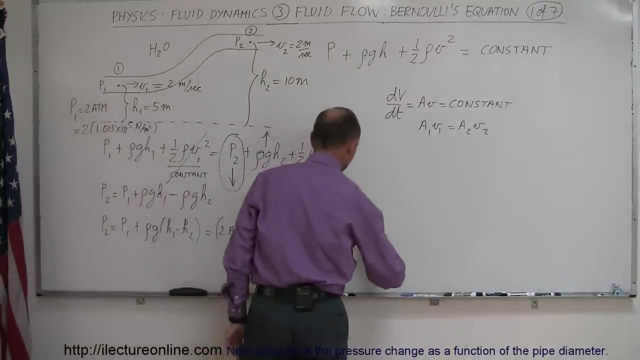 square meter. so one thousand kilograms, not per square but per cubic meter, of course, because it's per volume. g is nine point eight meters per second square, and then we multiply that times h one minus h two. now h one is five meters, h two is ten meters, and so very quickly. 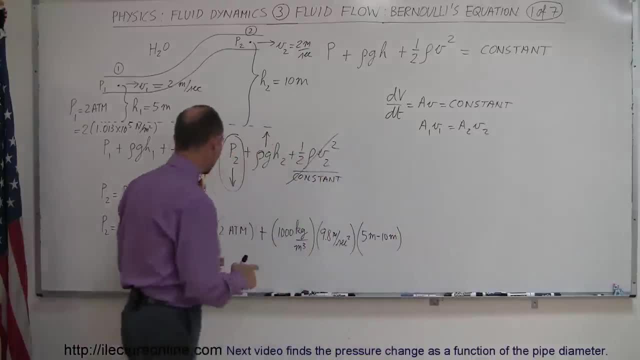 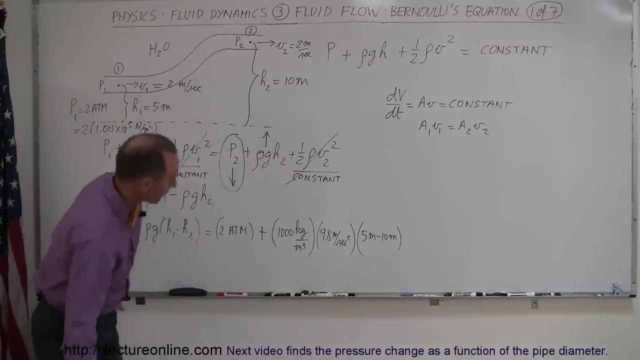 you can see that that would be a negative number, which means that the pressure will be less. and so at point two, compared to point one, now how much less? all right, let's find out. so that would be one thousand times nine. point eight, that would be nine thousand eight hundred. 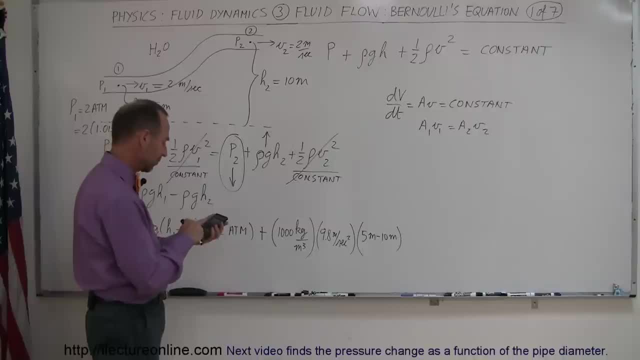 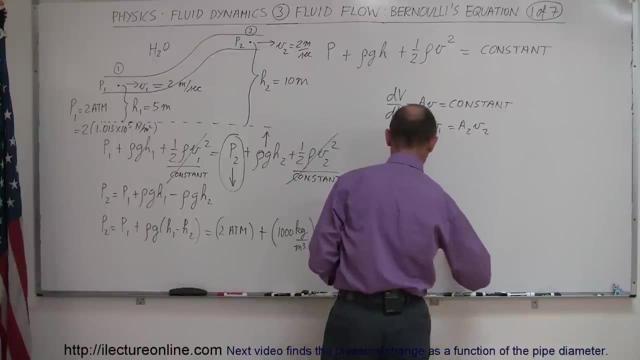 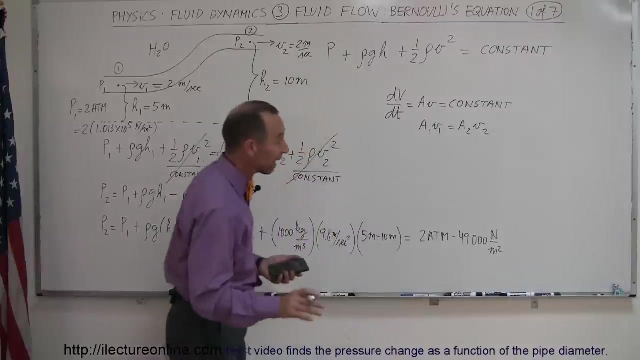 times five minus ten, which is minus five. so times five equals that's forty nine thousand. so this is equal to two atmospheres minus forty nine thousand newtons per square meter. now there's a unit for that. we call pascal, so you can say: pascals are newtons per square meter. 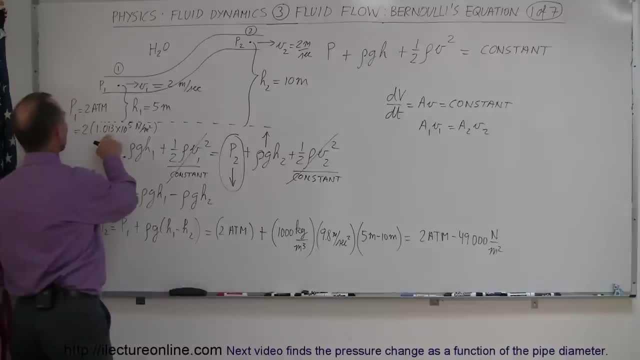 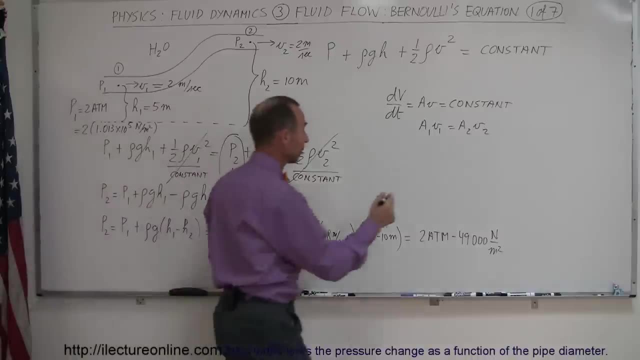 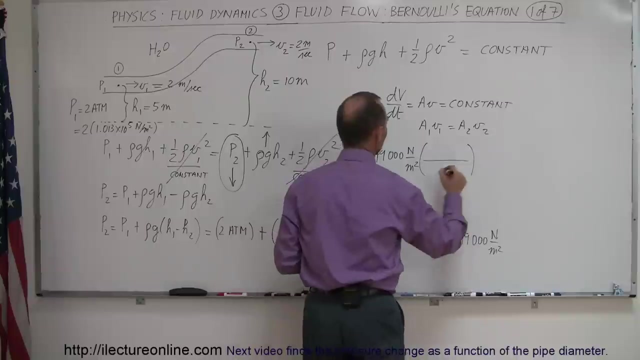 now, if one atmosphere is 101 300 newtons per square meter, what is 49 000 newtons per square meter in terms of atmospheres? so let's do that real quick here. if i have 49 000 newtons per square meter and we convert that to atmospheres, so one atmosphere is equal to 101 300 newtons per 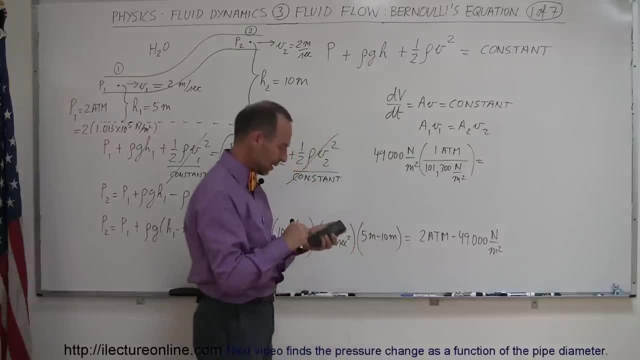 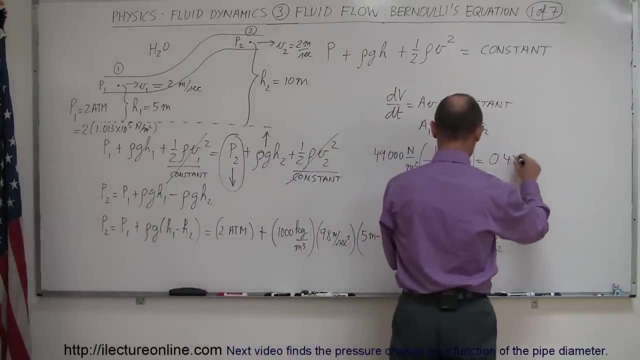 square meter. so we can see: if we take that divided by 101, 300, one too many equals and that would be 0.48 atmospheres. all right, so this can then be written as two atmospheres minus 0.48 atmospheres, so we can say this is equal to 1.52 atmospheres. there we go now quickly looking at again.